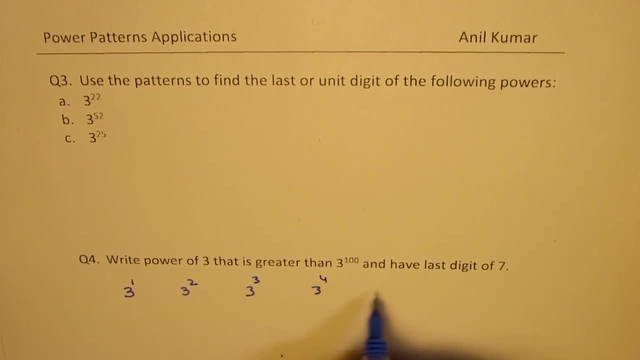 3 to the power of 5.. 3 to the power of 3,, 3 to the power 4, ,3 to power 5,, 3 to the power 6, and so on. So well, 3 to the power of 1 is three. number itself times 2,. 3 to the power of 2 is. 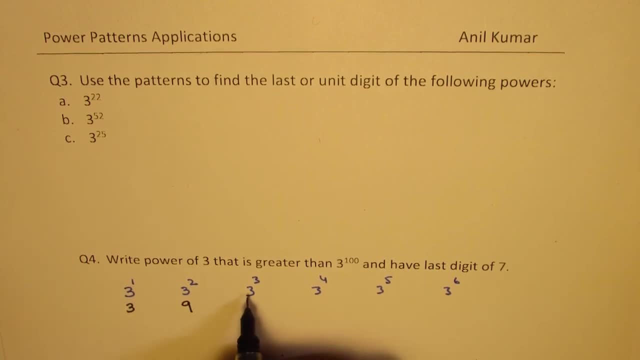 three times 3, twice. you multiply it with 9. 3 to power 3 is 27, so you can multiply the previous number by 3 to get the next power. there is to get 81 here. multiply 81 by 3 to right here you get 83.. 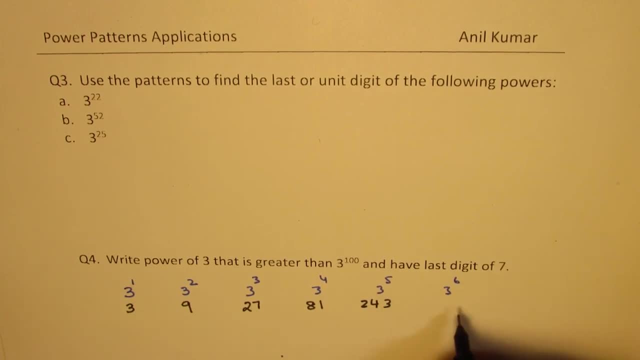 24 x 3, 3 times 3 is 3 times 3 is 9, so we get 9 here. and 3 times 4 is 12, 2 and 1, 729 and so on. so what you really notice at these powers, the place value, is what? 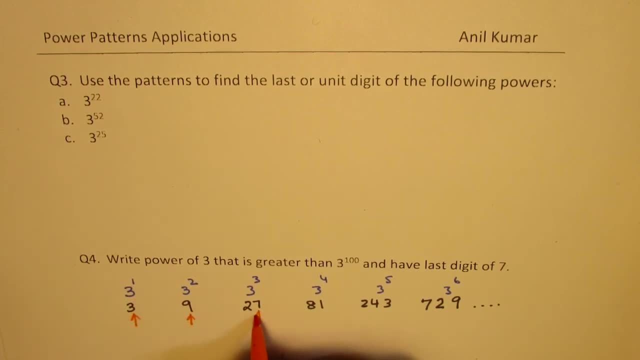 so place value is 3, 9, 7, 1, and then again this set of values repeat. we again have 3, 9 and if you continue, this pattern repeats. okay, so from this pattern rule, or we can say in general that if I have 3 to the power of n, right, and if I 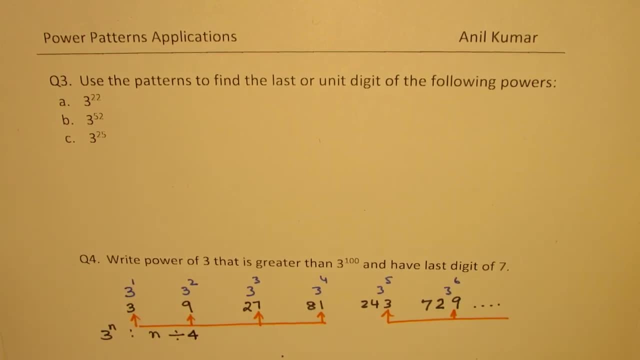 divide n by 4. in that case remainder will decide the units digit. is that clear to you, right? so dividing by 4, if the remainder is 1, then you get 3 as your unit state. if the remainder is 2, then the unit stage it will be 9 if it. 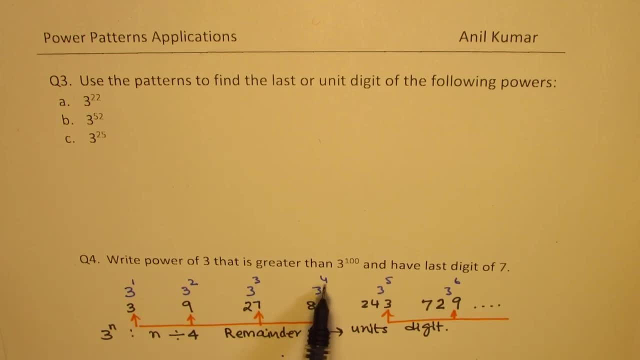 is 3, it will be 7. 4 means it goes evenly. remainder is 0: right, then you get 1 as your answer, correct. so so basically, if we have, we can now write the rules. if the remainder could be 1, it could be 2, it could be 3 or it. 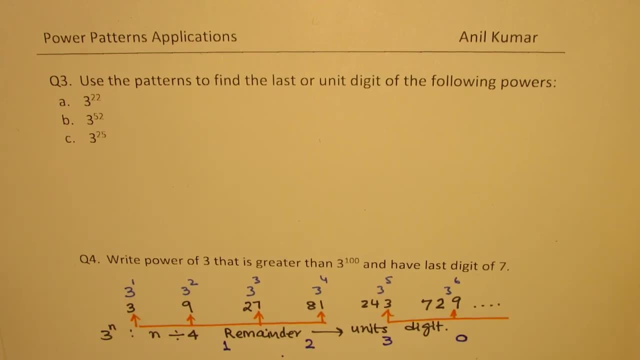 could be 0. you could have written 0 in the beginning also, but we're just following this pattern. so if it is 1, the units place will be 3, if it is 2 units place will be 9, if it is 3 it will be 7, and if the remainder is 0, then it is going to. 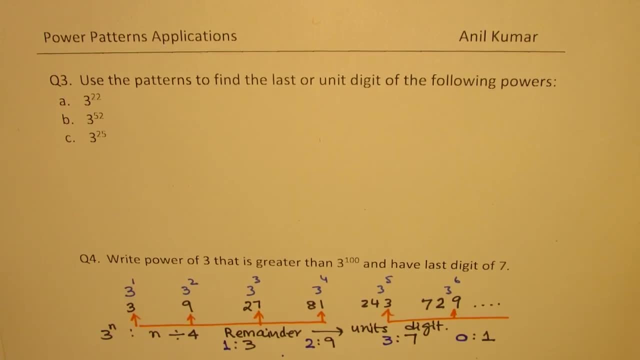 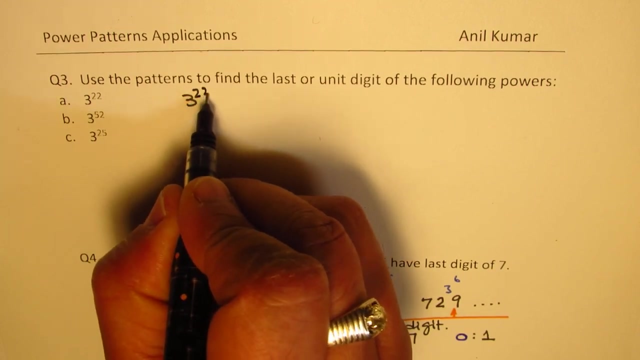 be 1, like 3 to the power of 0 is 1. does it make sense to you, right? okay? so now, using this pattern rule, let us answer our questions. so let's begin with: 3 to the power of 22. so 3 to the power of 22 will actually divide 22 by 4, right? 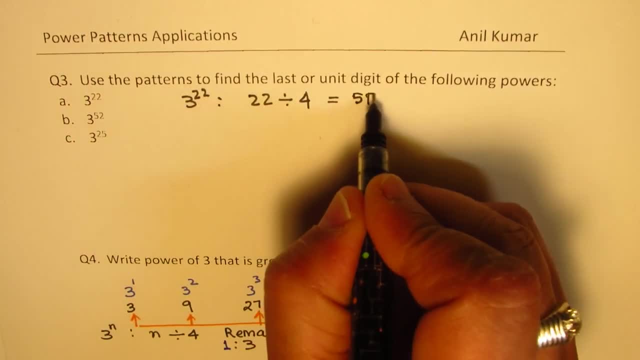 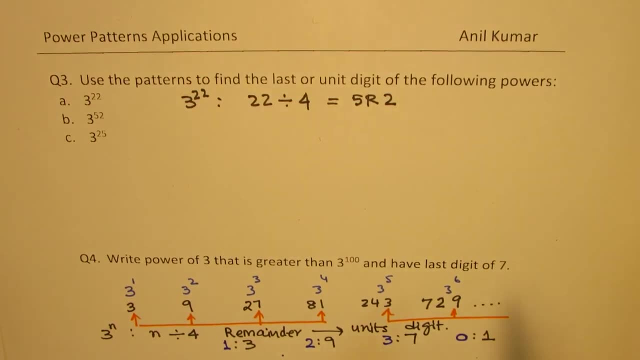 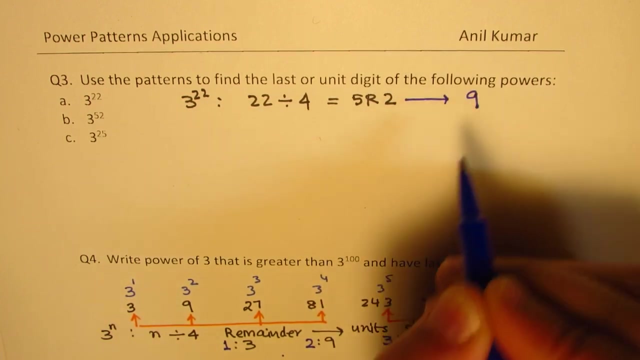 so when you divide 22 by 4, it goes 5 times with the remainder of 2. now, since the remainder is 2, what is the units place? well, if the remainder is 2, the unit place is 9, so this corresponds to units place of 9. clear that number 2 corresponds to unit. 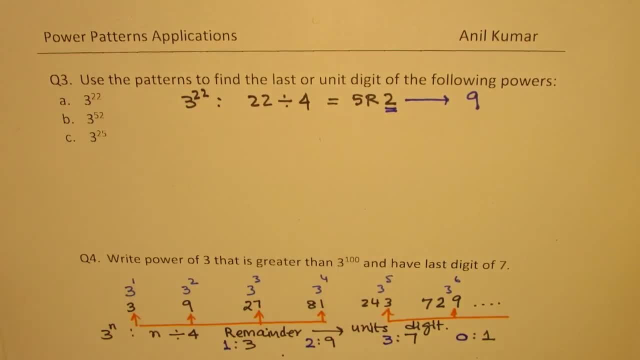 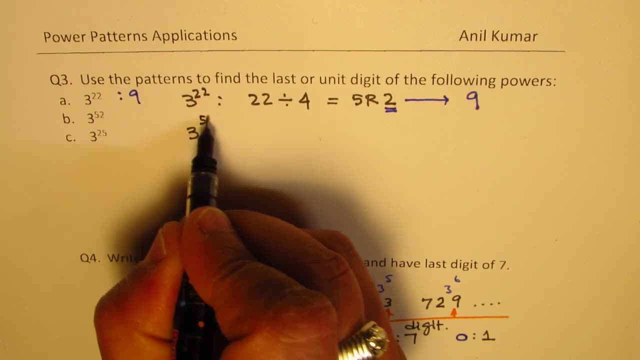 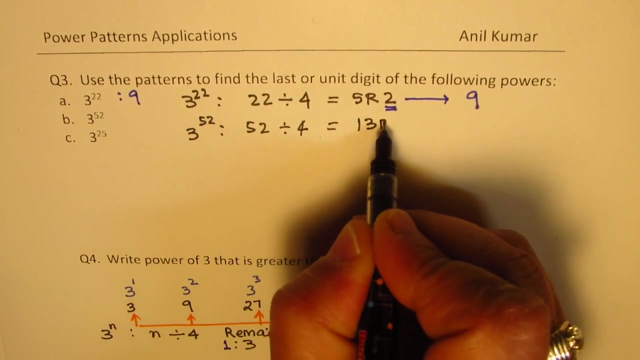 place of 9. so we get our answer here and that is going to be 9 for the first case. in the second case we have 3 to the power of 52. so let's again divide 52 by 4 and we go 1 and 3 13 times. remainder is 0. now, since the remainder is 0, we get. 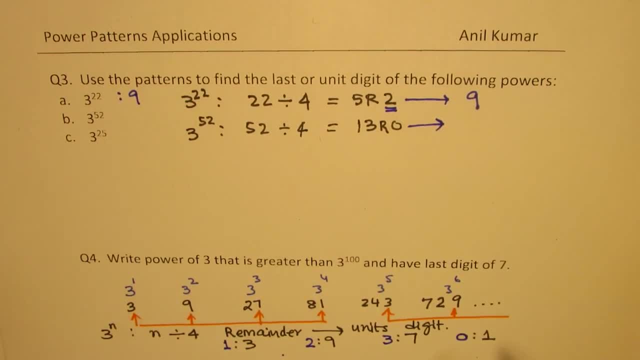 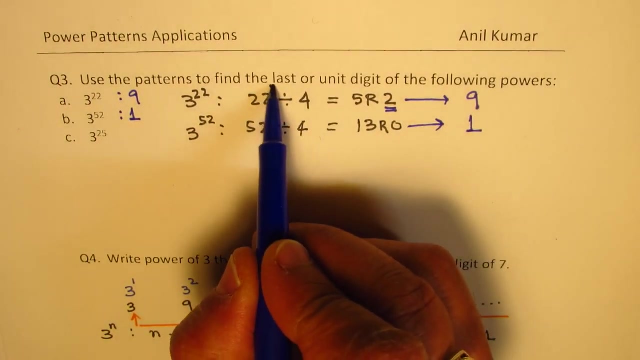 power as 1. correct, as mentioned here. so it is going to be 1 and this remainder the ones place, or the last digit or the unit digit will be 1. so this question could be asked in different ways. sometimes we say last or once or unit digit. correct the C part. 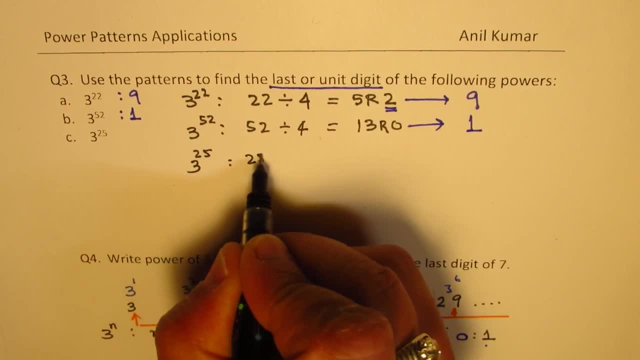 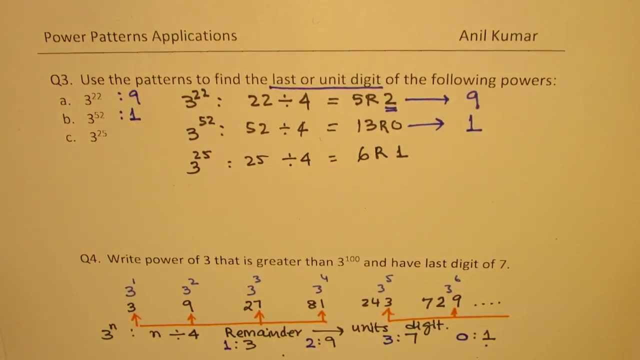 is 3 to the power 25. so if I divide 25 by 4, we get what? 6 times 24 and remainder is one and for remainder one it is three, Clear. So here the remainder is three. That is how we could answer the question. Now, question number four here is write powers of three. 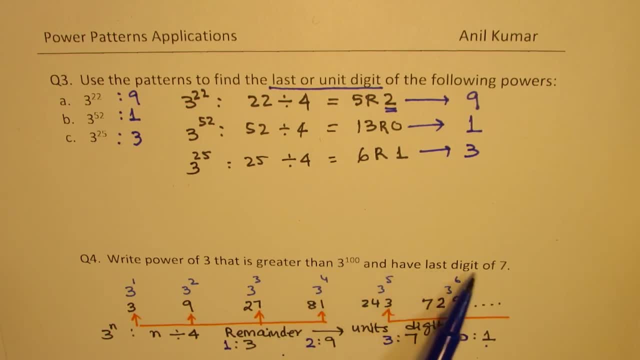 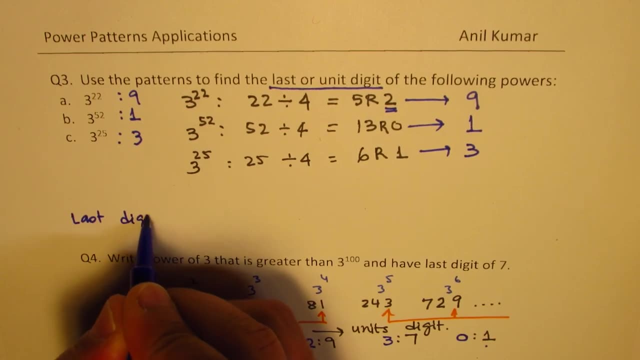 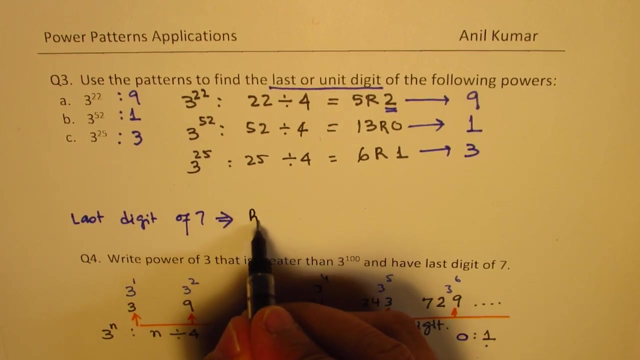 that are greater than three to the power of hundred and have last digit as seven. So last digit of seven means what? It means that the remainder should be three, right? So we are looking into this portion remainder being three, We know, three to the power of hundred.